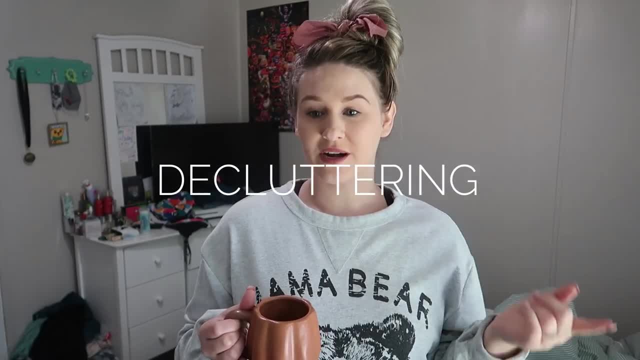 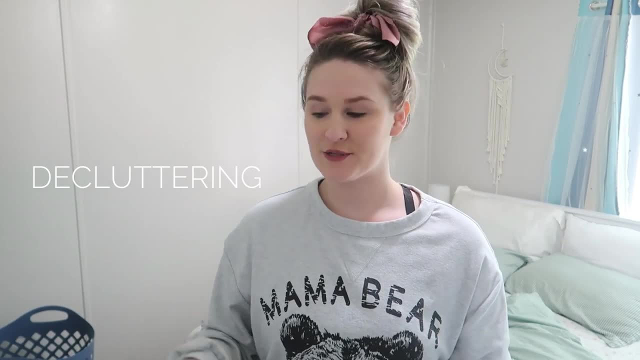 I'm going to go ahead and get started with decluttering, organizing and cleaning this room. So I have two trash bags: One's going to be for trash, One's going to be for things that I'm trying to declutter out of this room. I have my peachy keen monster, because it is much needed. 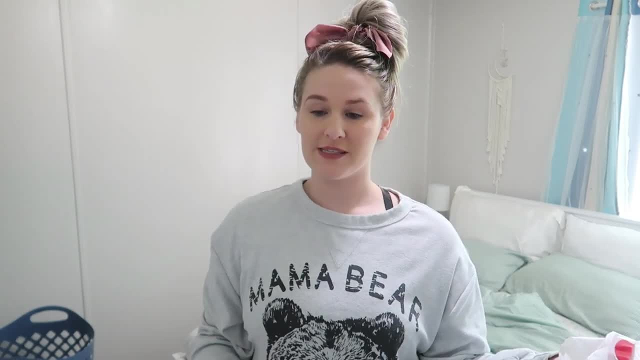 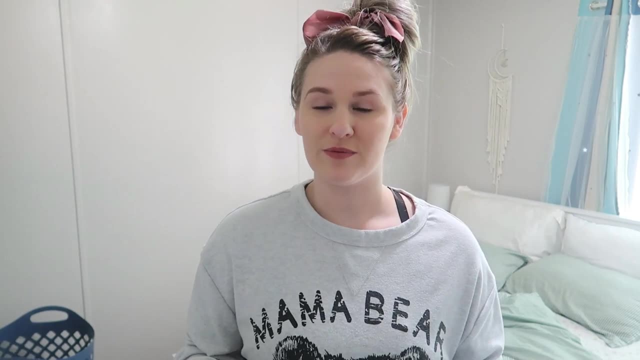 to tackle this room to get through this day. The boys are home with me. The girls are at school, Jackson's taking his nap, Nolan is doing some quiet time. He's actually eating lunch right now at the kitchen table. So I have about two hours until Arabella gets home. 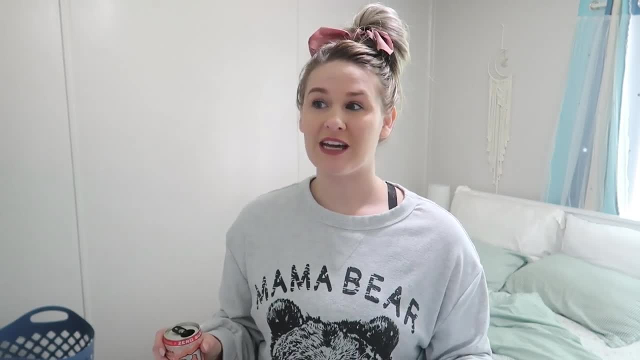 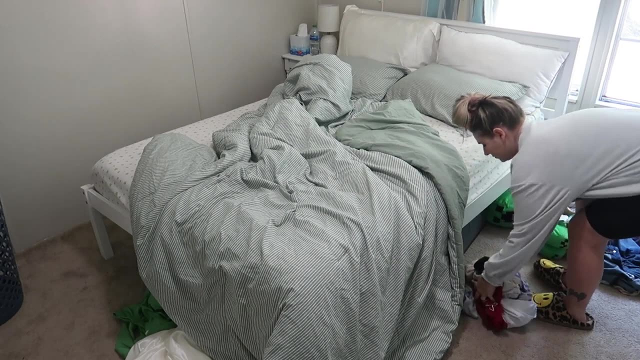 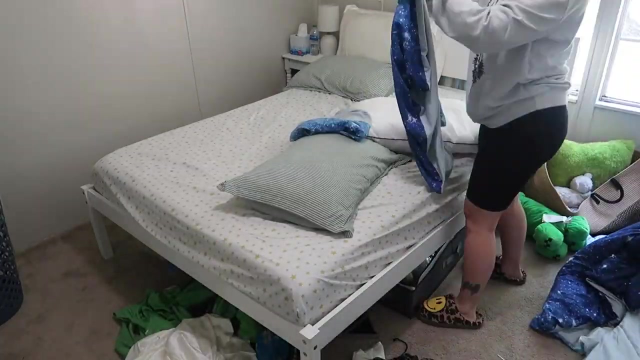 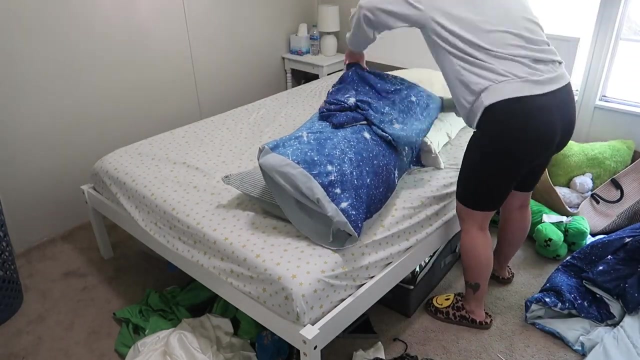 from school. So I'm going to try to do this in two hours. Fingers crossed I can get it done. It's going to take a lot of speed cleaning, So, cheers, The first thing I'm going to do is go ahead and get her bed made up, because 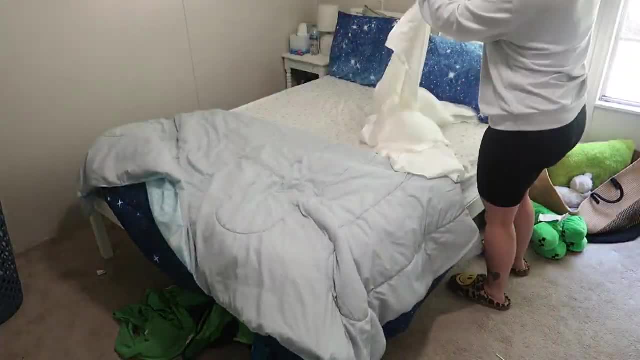 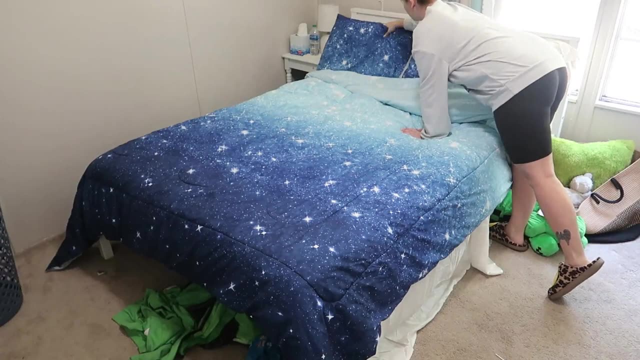 making up the bed already makes the room look 10 times cleaner, And that way I can pile things on her bed without it getting lost in her blankets. So I'm going to put her silk sheet on her comforter, get her pillows all made up, And then the next thing I'm going to be doing is 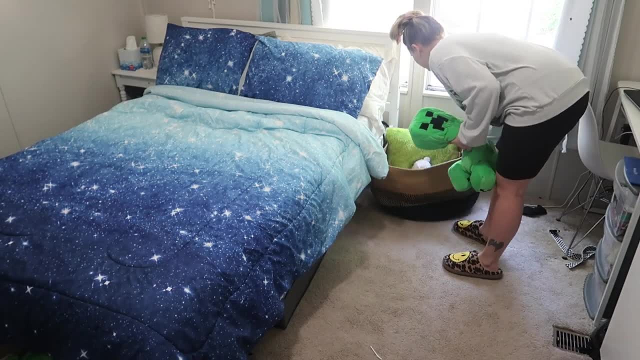 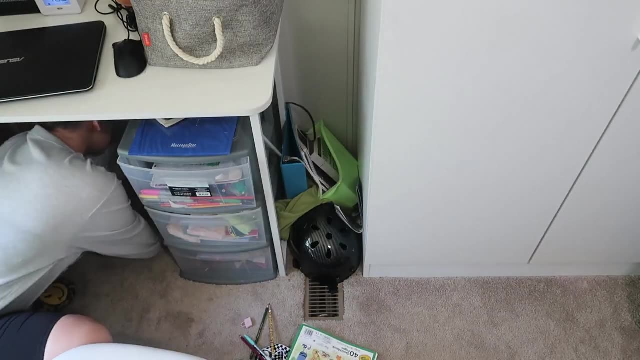 making piles on things that I'm going to be keeping, things we're going to be decluttering, And then I'm also going to be cleaning along the way. It's always so overwhelming whenever you walk into your kid's room and it looks like this, So my tip to you is to focus on one corner of the room. 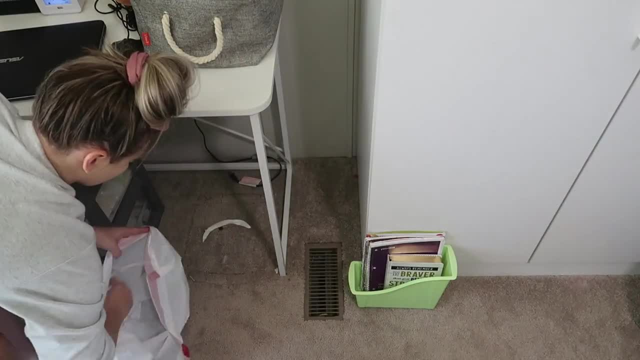 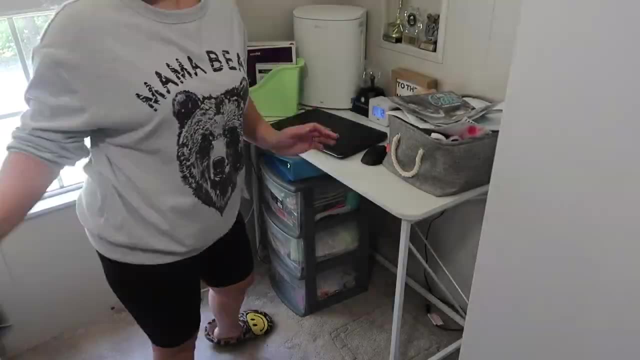 over here in her desk area. So the first thing I'm going to do is declutter the top of her desk. I'm going through all her papers. She has little notes that her friends had wrote her And some things you could just tell was just trash, And so I'm just going to go through here, declutter stuff. 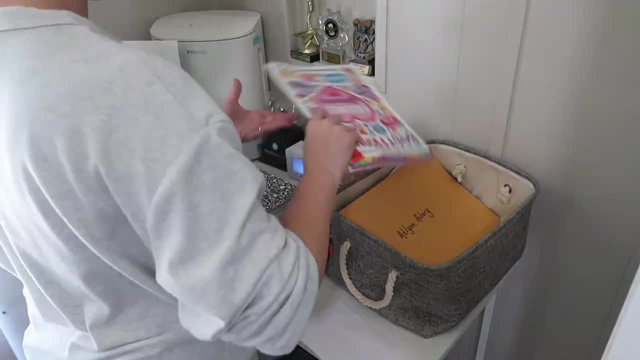 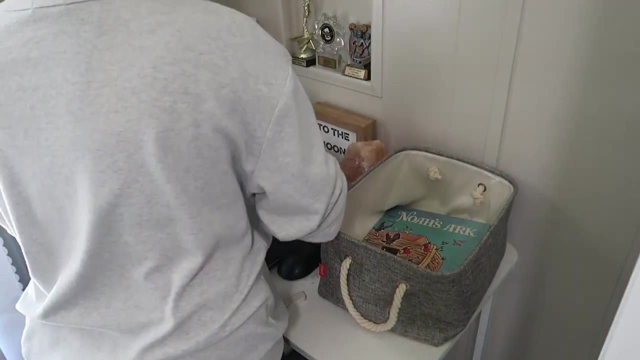 Again, I'm going to be putting everything in the kitchen for her to go through whenever she gets home from school so she can decide herself if she wants to keep it or not. But I went through everything and I decluttered broken pencils, pencils that didn't have erasers, And I really 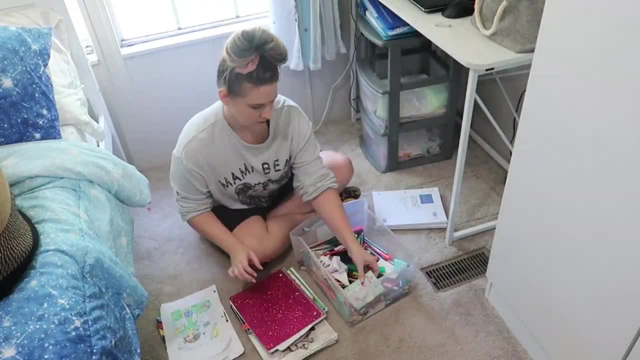 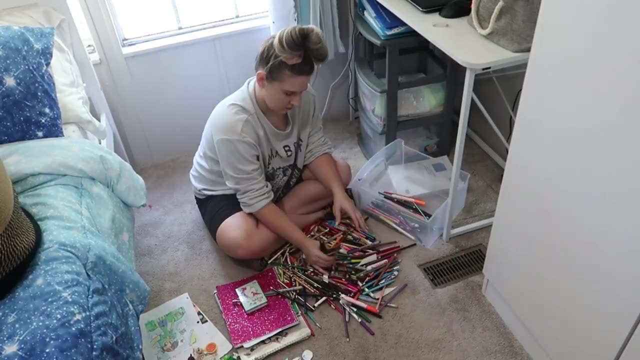 really didn't want to dump this out y'all. I really did not want to dump out all of the colored pencils in the floor, But there was so many pieces of paper in it, it just really needed to be dumped out. So it felt so nice to have that tackled and taken care of, decluttered, And then she had all. 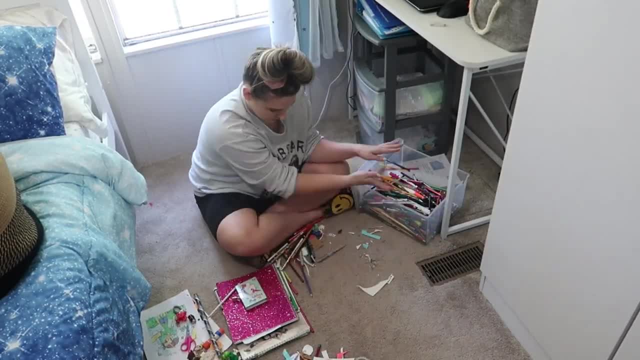 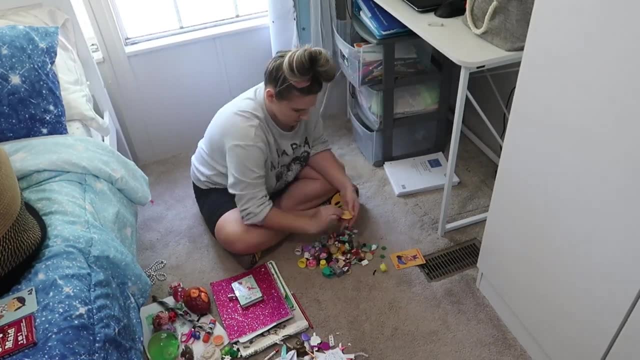 these tiny little toys, So some pieces were broken. I just went ahead and threw those away And I put everything back in there for her to go through. So she is going to go through her room one more time when she gets home and declutter anything extra that she may find. But I think I 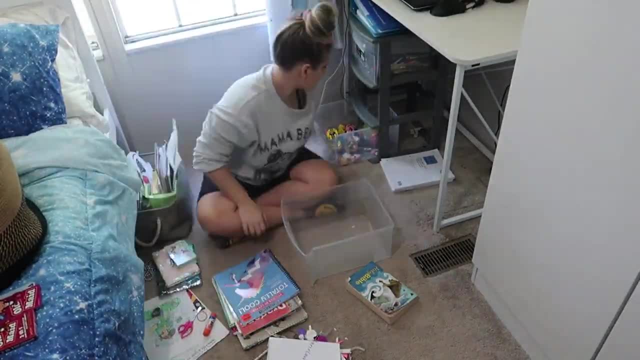 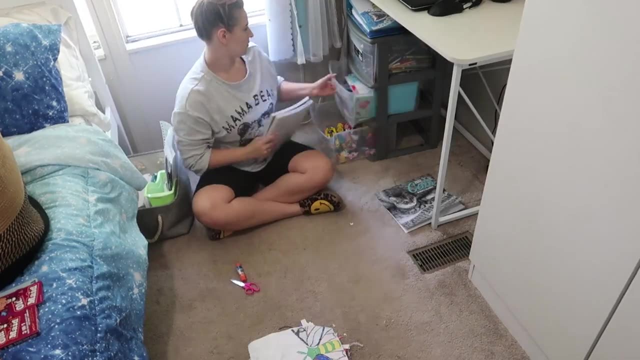 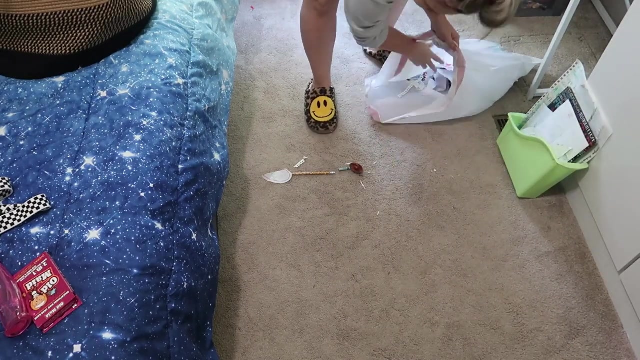 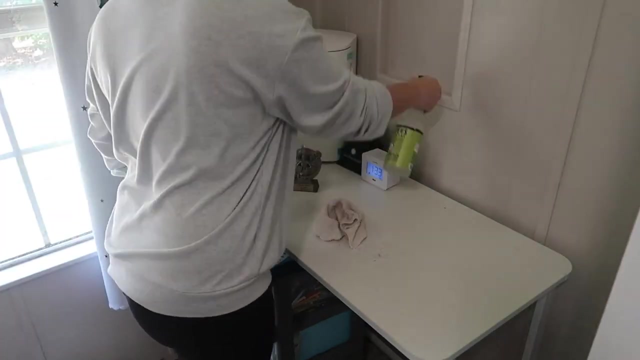 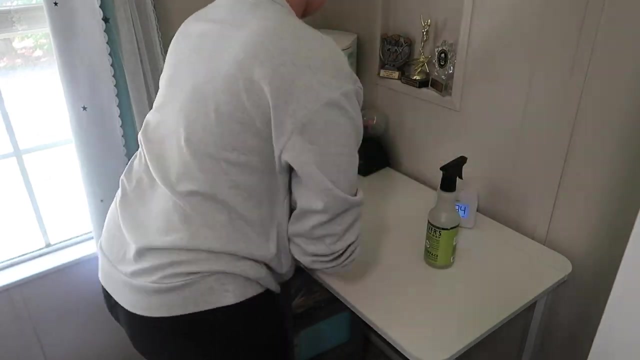 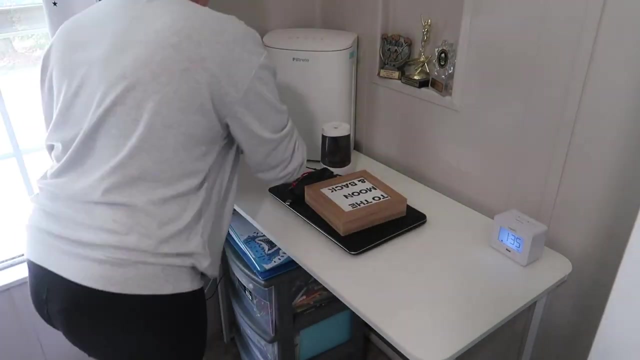 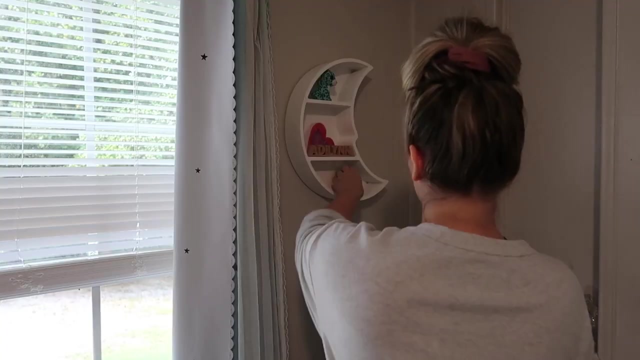 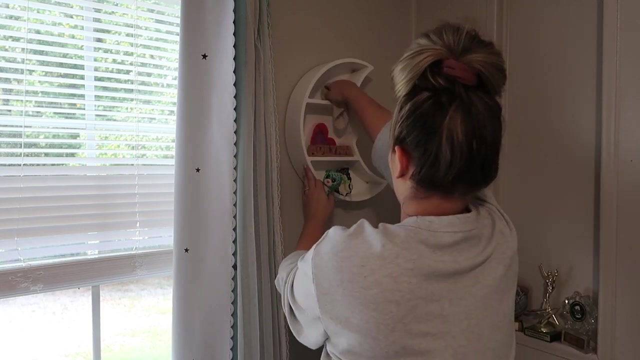 did a really good job in the end. I'm going to be doing a tour At the end of this video to show you guys the way that I ended up organizing her room. Okay, let's talk about this shoe situation. Most people have closets to put their shoes in. 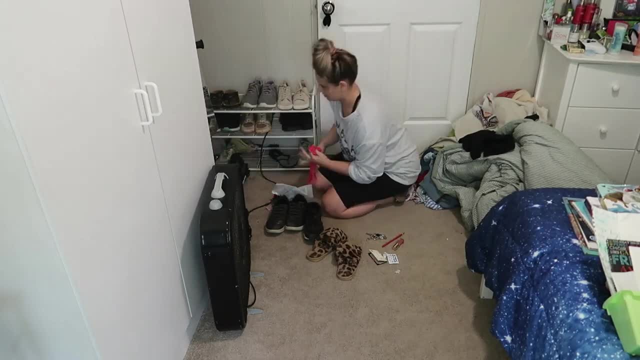 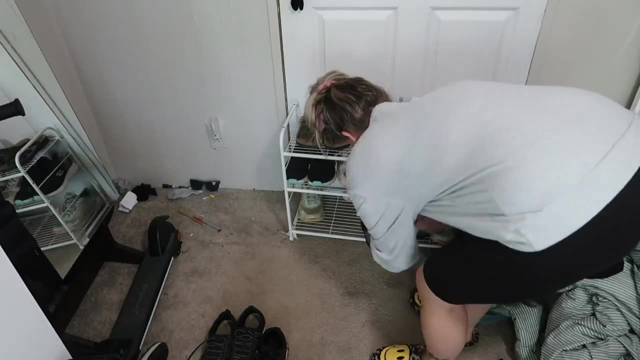 right? Well, this room does not have a closet, So I have the what we call wardrobe closet here that we purchased from Lowe's, And that's where I keep all of her clothes, And I don't like to keep her shoes in there. Originally, I had her shoes in it. 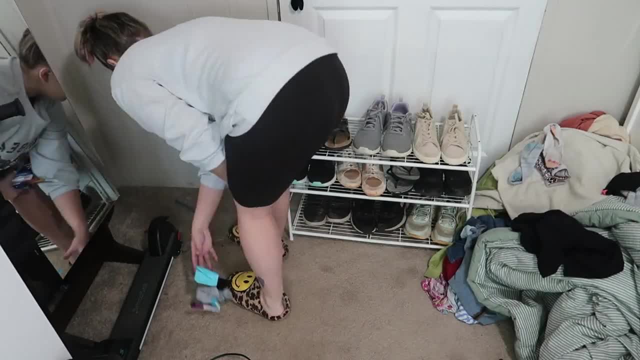 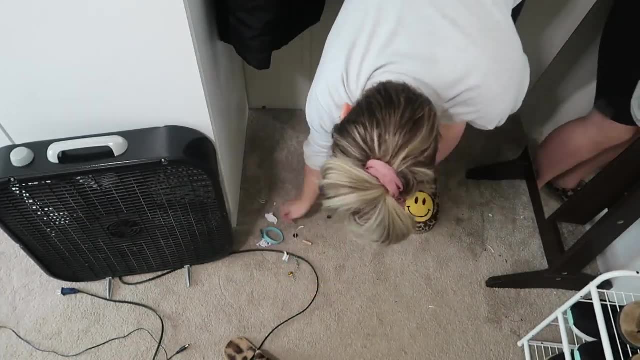 And it honestly made the closet smell like stinky shoes. So I just purchased this shoe bench that I keep over here in the corner for her to put all of her shoes on, And you never know what you're going to find. in a kid's room, I literally found Sandy from 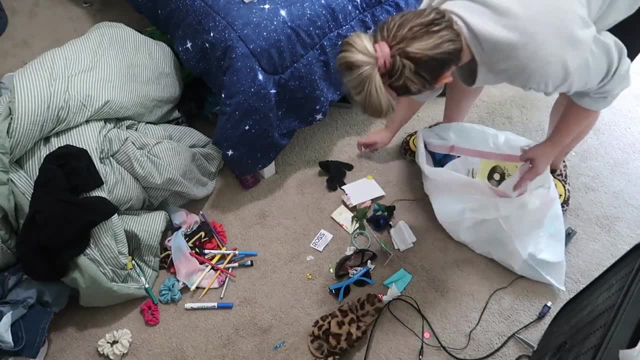 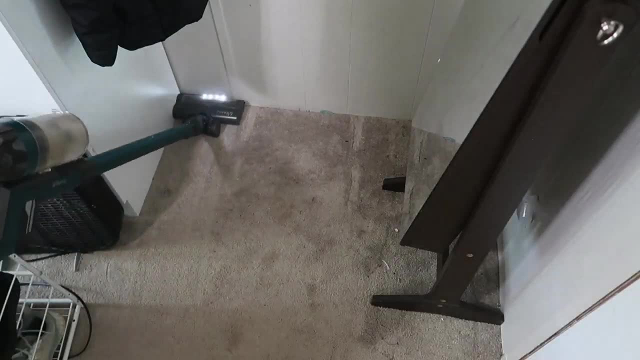 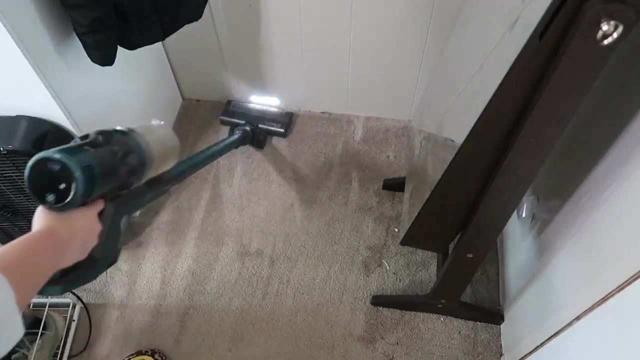 treasure box thing or something. So she always gets like really super random toys like that. The other day she had a penguin and she named it like Mr Charles or something weird And we went to Dairy Queen and she sadly left it there. So she did lose that. she was kind of upset about it. But 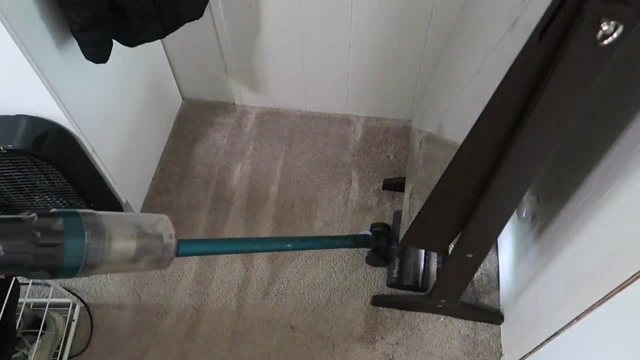 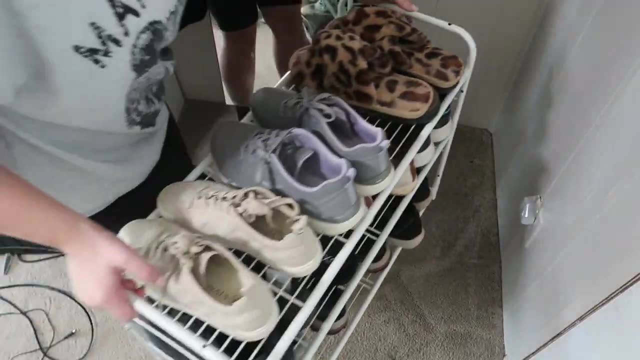 I just find the weirdest little things in my kids room. So there is little pieces of paper everywhere because Adeline is an artist. She is always hard at work making masks and making all kinds of projects in her room. So there was so many shredded up pieces of paper all around in her room And I 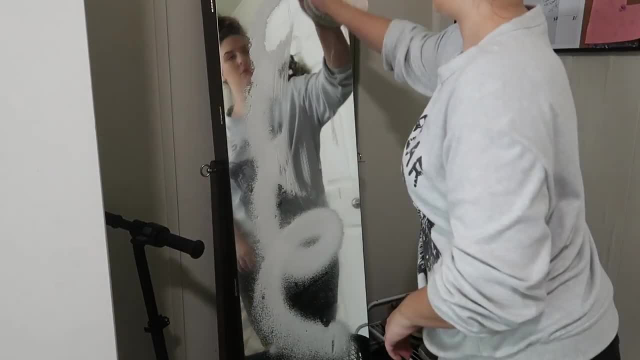 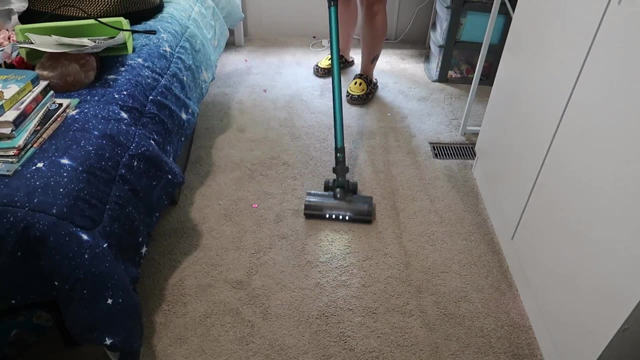 keep her electric scooter in her room, because we live in a mobile home So we obviously don't have a garage or anything like that. That would be so nice if we did, But I just have to store things like that in my kids room. So underneath her bed I end up storing her skateboard. I do have an. outside storage building where we put like their regular scooters. but I didn't want to put her motorized scooter out there and risk it getting damaged, And she charges it in her room anyways. It's not the most ideal way to store a scooter, but that's what works for us. 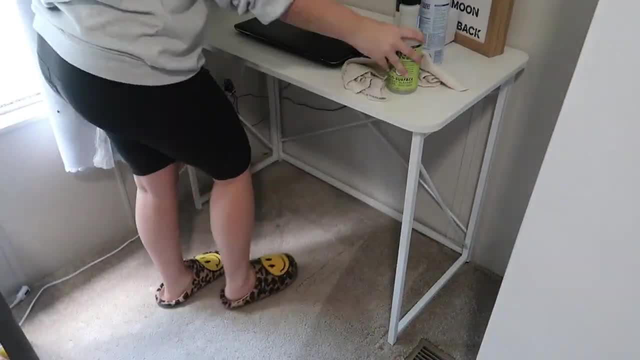 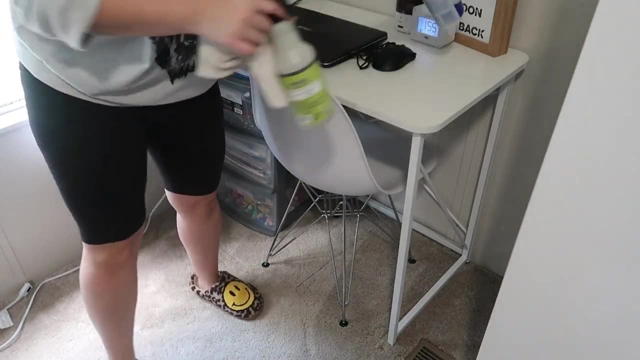 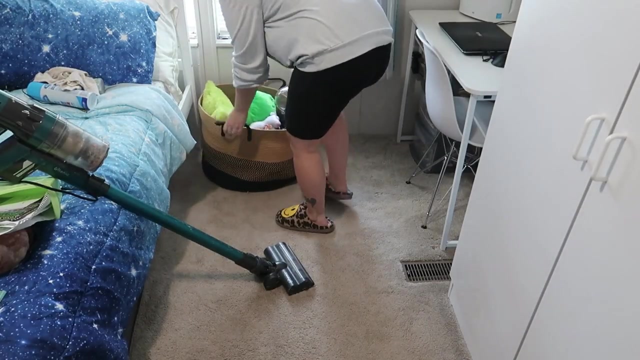 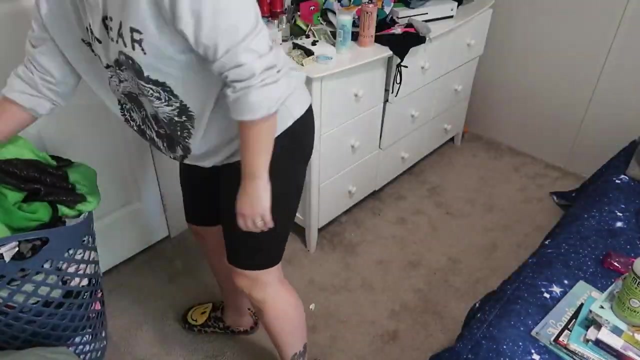 Y'all. that was clean laundry and dirty laundry everywhere. So I just went ahead and put all of the laundry in the basket and we're just going to go wash all of it. And here is the cutest little crown that Adeline made. She made it for one of her stuffed animals and she put tape on it so that 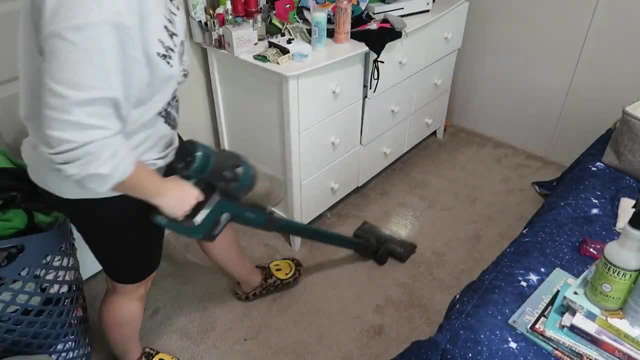 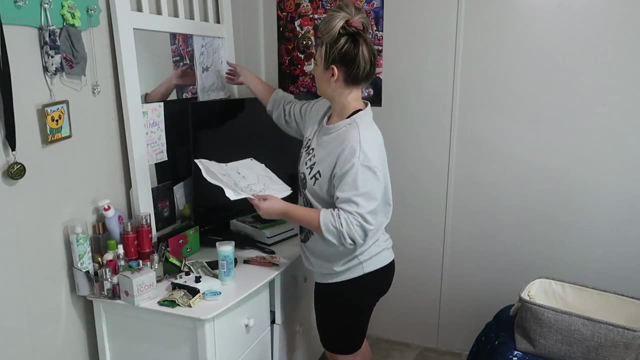 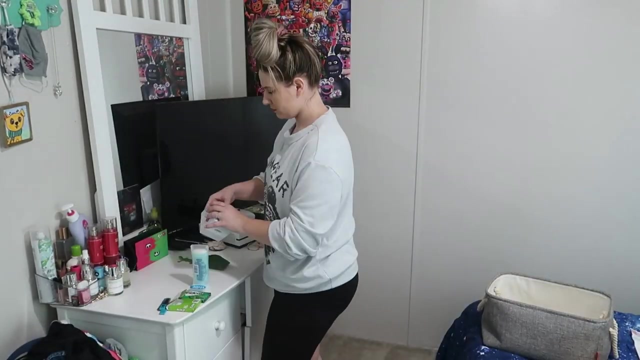 she could use it for her laundry. So I'm going to go wash all of it. And here is the cutest little: the stuffed animal's head. So I just love finding little things like that in her room. I think it's so precious. A dresser naturally just becomes a catch-all and her dresser is obviously overdone. 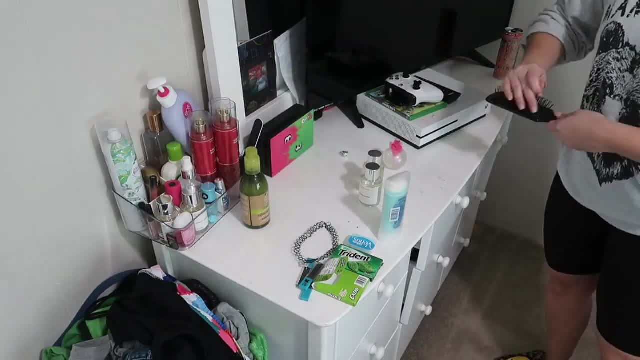 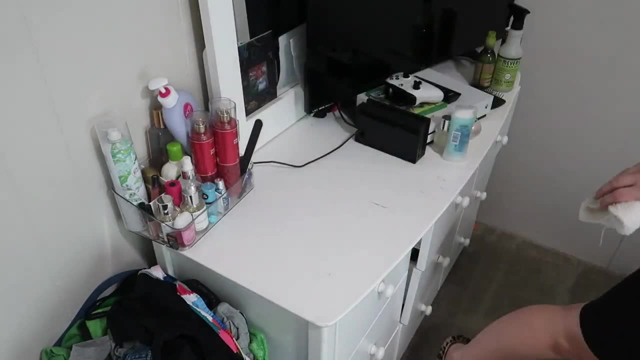 in a catch-all. There is crap everywhere, So I'm going to be wiping it down. It was quite dusty and this little organizer y'all is from Target Dollar Spot for $5 and I love it so much. I need to find some kind of organization deal for her lotions and her perfumes other than sitting them. 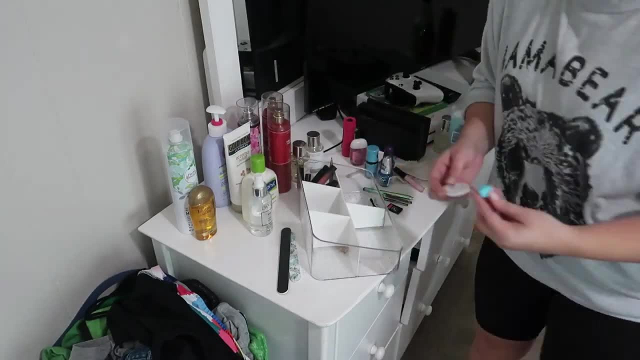 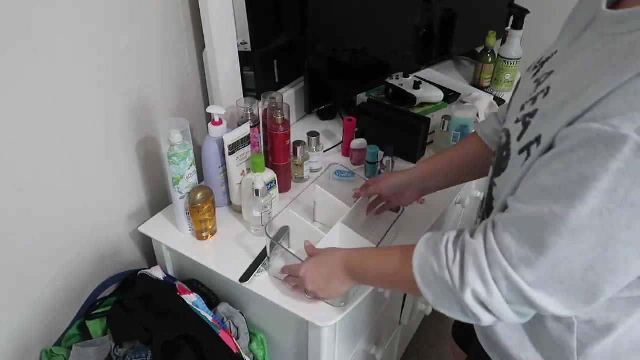 in the closet, because I already tried that and they ended up just getting flipped over and knocked around. So I need to get some sort of basket or something for all of her lotions. But as far as her like lip gloss and nail polishes and things like that, I keep them in this little. 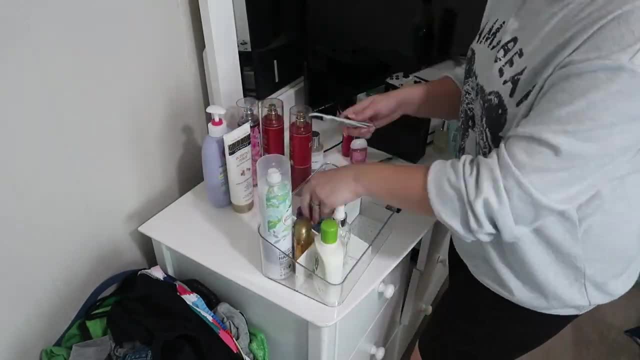 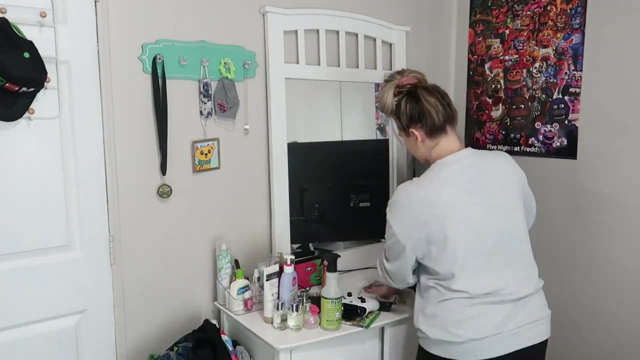 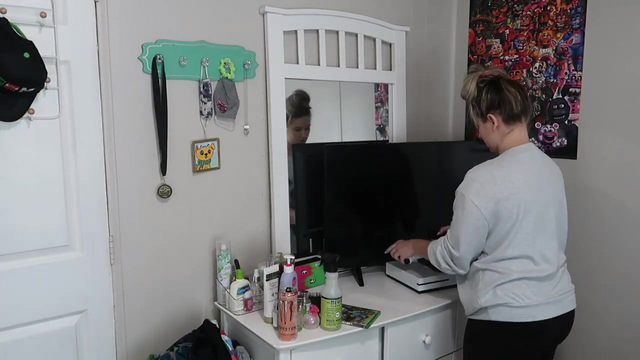 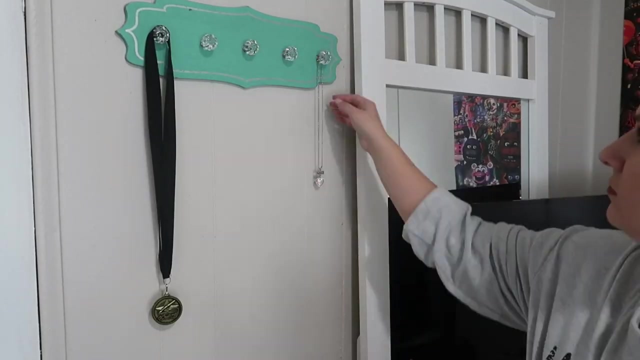 storage caddy. I would love to hear your ideas, if you have any ideas for me on how to store her lotions and things like that. The next corner I'm tackling is her wardrobe, which is her closet, So this is where all of her 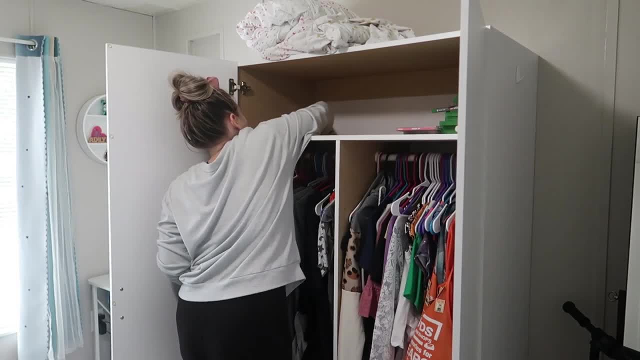 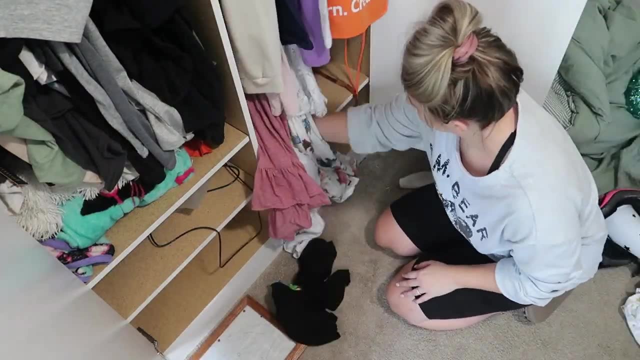 clothes are And, as you can see, her games and CDs and everything was just a huge mess in here. So I'm going to be wiping it down. I'm going to store her books in here- This is some Legos- and then I'm actually going to be moving her games over to her desk here in just a minute. 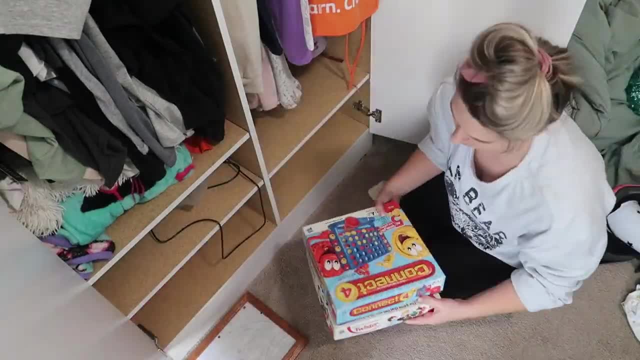 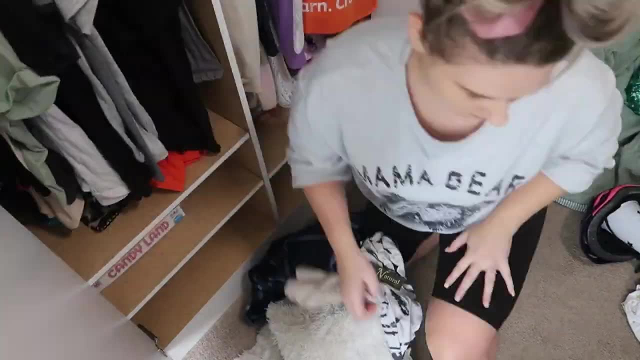 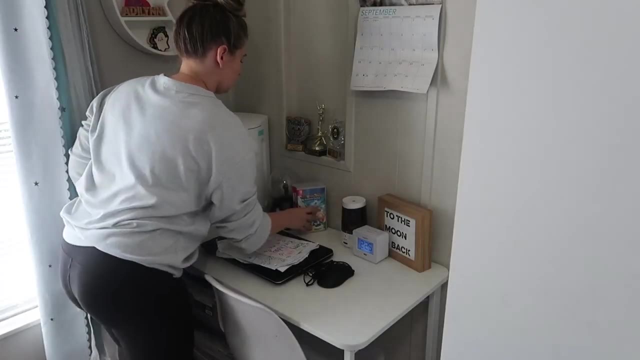 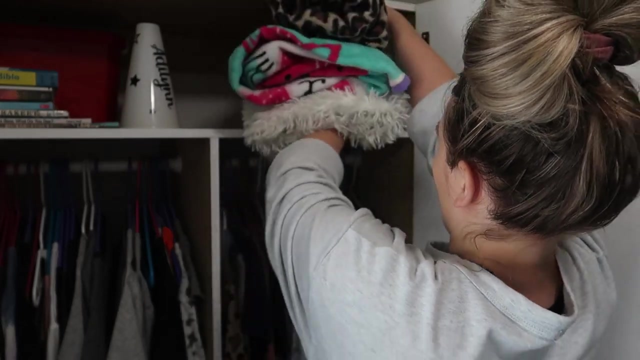 So I'm just going to be wiping down all the shelves, and under here is not really cluttered. I just keep some board games under here and just some keepsakes and her personal items. things like that stay in her closet, So she has extra comforters and sheets and pillowcases, So I thought that I would go ahead. 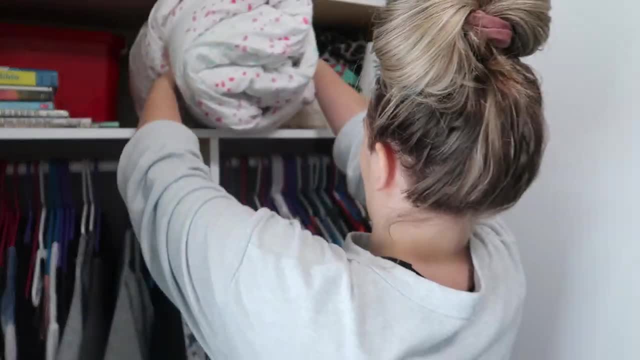 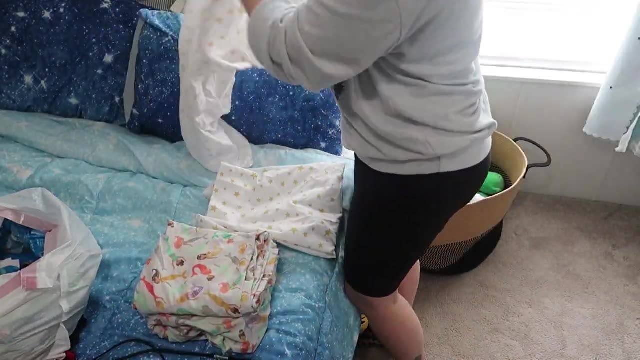 and store those up here in the top of the closet. Sometimes she has friends come over and spend the night, So it's all good. So I'm just going to be wiping down all the shelves and under. here is nice to have extra blankets and extra pillowcases and just clean laundry for company, And I don't. 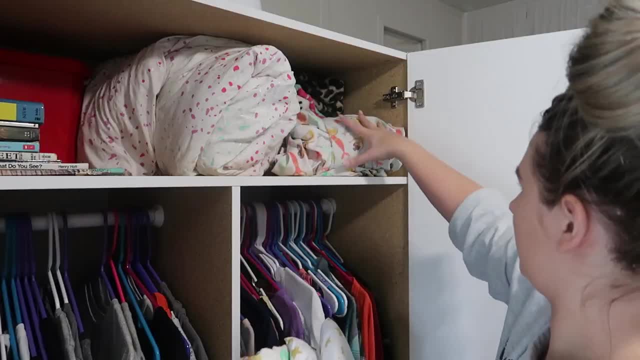 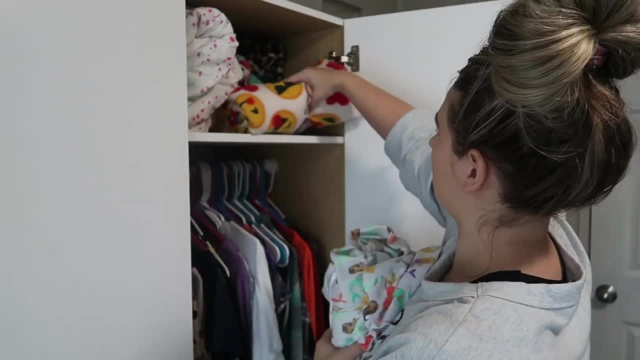 know what I would do if we did not purchase this wardrobe closet, because she has so much stuff in this closet. I don't know what I would do without this thing, And next I'm going to go ahead and make piles on her bed of all the little stuff. So I've just kind of been using her bed as a table. 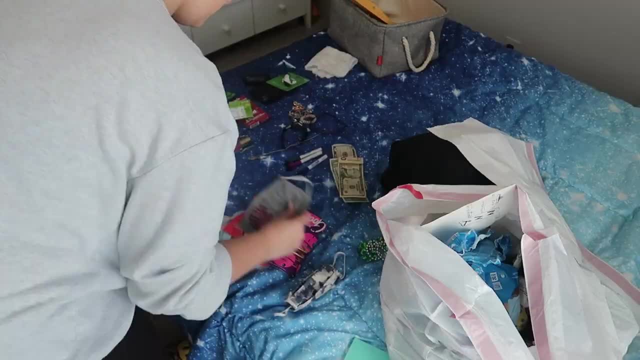 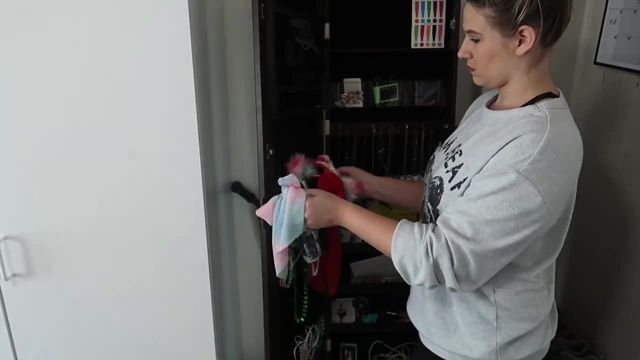 to just put stuff on. So I'm categorizing everything from jewelry to makeup to headbands and just where everything's supposed to go, And that makes it so much easier, Whenever I go, to put everything away, so I don't have to make 50-11 trips. 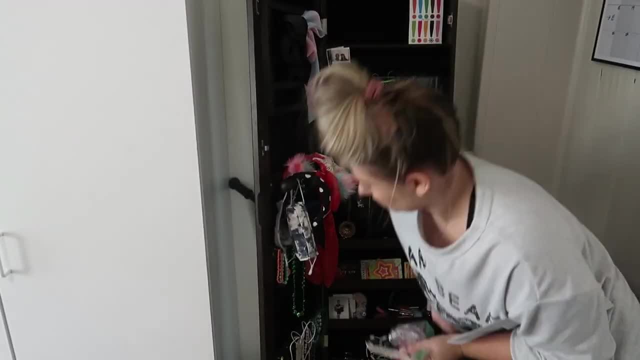 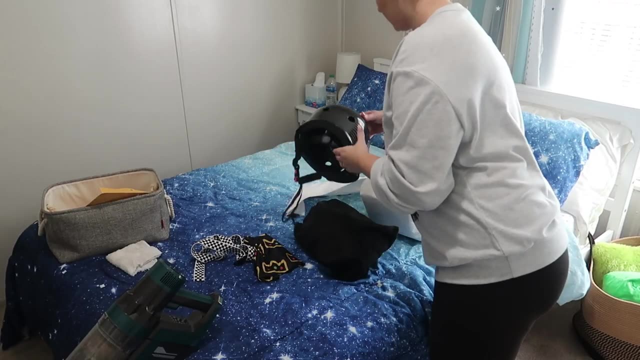 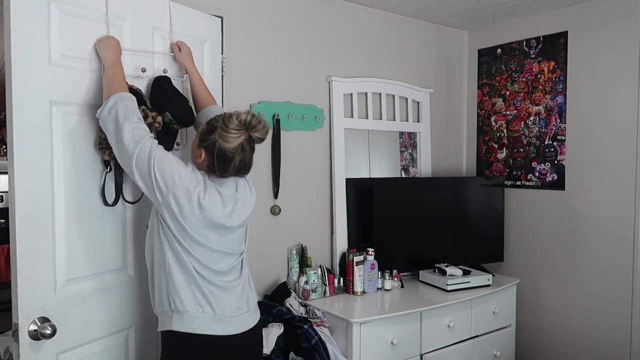 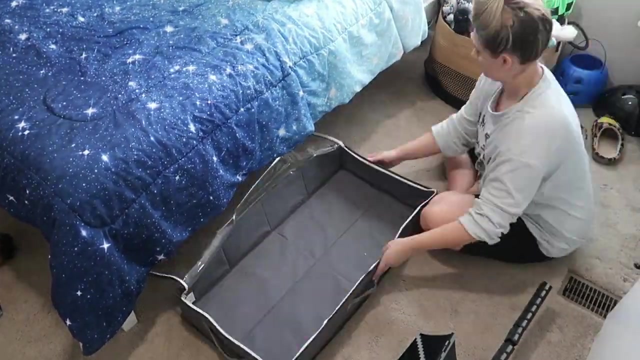 I can just take all the hair bows and scrunchies and go put those up and then come back and get all the jewelry, put that up, so on and so forth. And for underneath the bed- as long as we have space under there, I utilize it to store things. So I have these under bed storage containers. 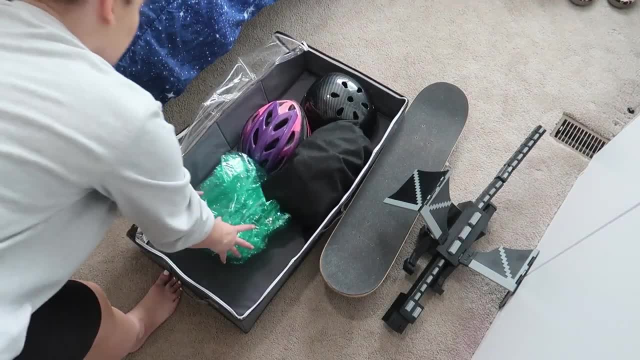 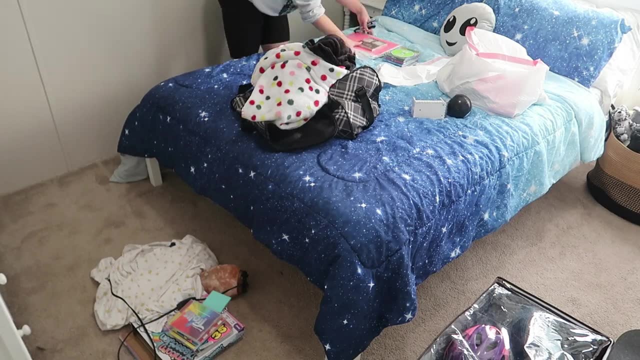 And this helps so much without having to just shove stuff under the bed. So I just have her bike helmet and her skateboard helmet- things like that- in here, And then I also have another tote that I'm going to be storing larger toys in, And then the little pile at the foot of the bed. 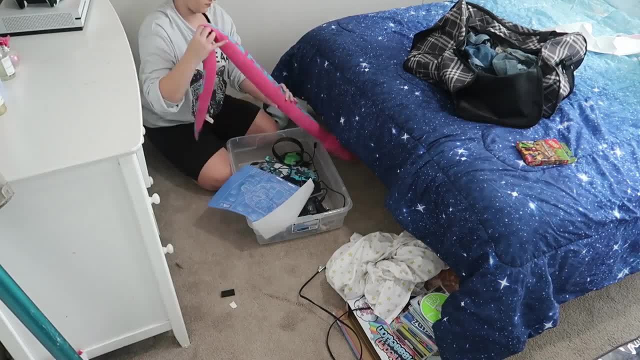 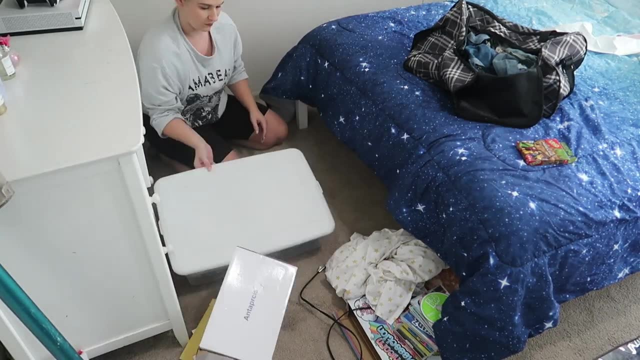 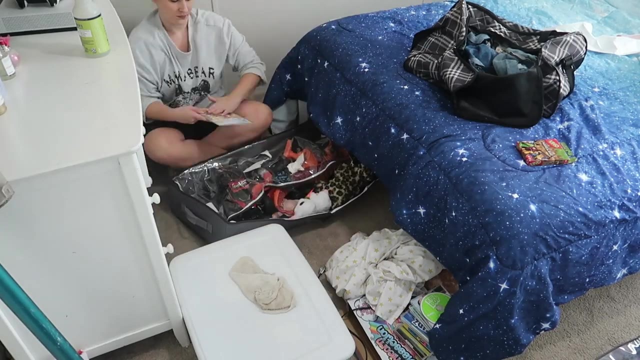 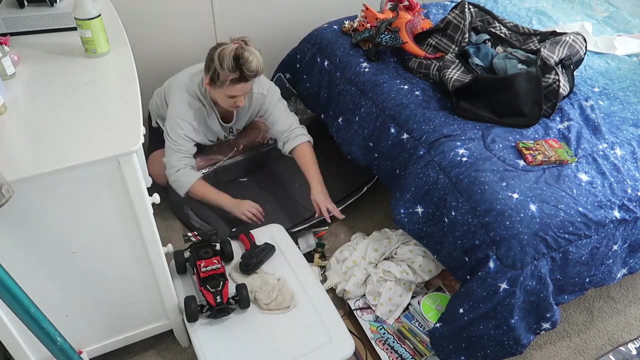 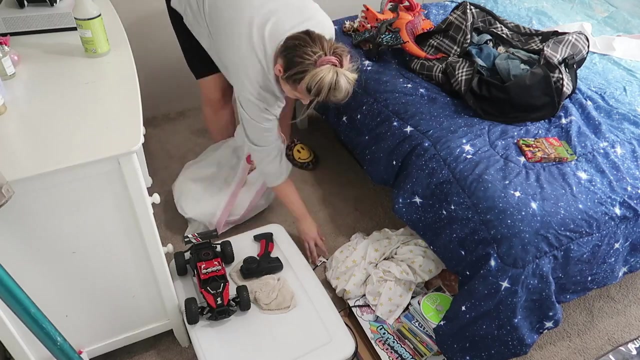 is things that I'm decluttering or passing down to Arabella or Nolan. It's amazing what you can find in a kid's room. There was just stuff everywhere. There was so much stuff that I found that just wasn't being used. So I passed down this remote control car. 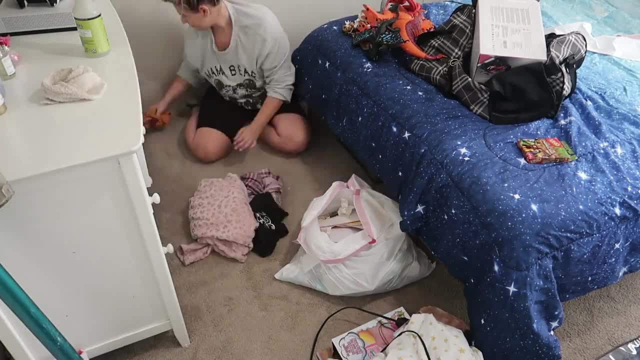 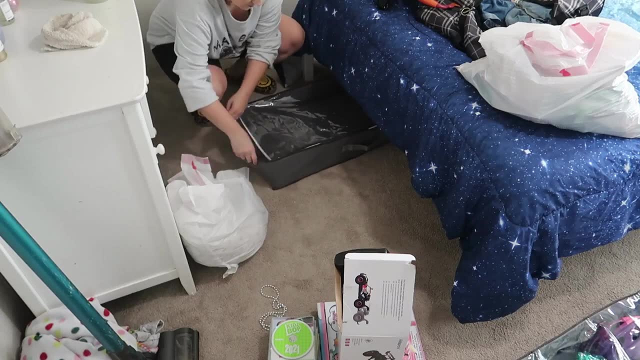 to Nolan, since Adeline never uses it. And then there was a unicorn game and all the Kidz Bop CDs that are getting passed down to Arabella. I also ended up with one trackbook trash bag of stuff that I can just get rid of and declutter and another trash bag that was just trash. 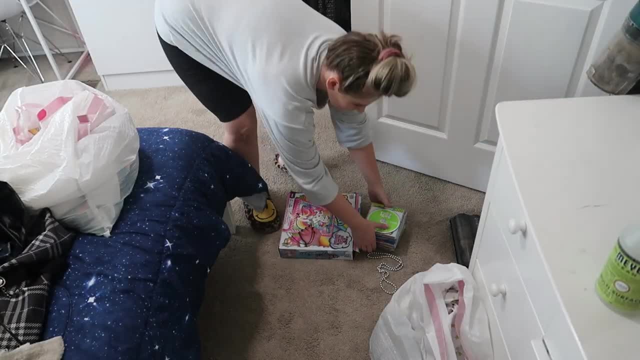 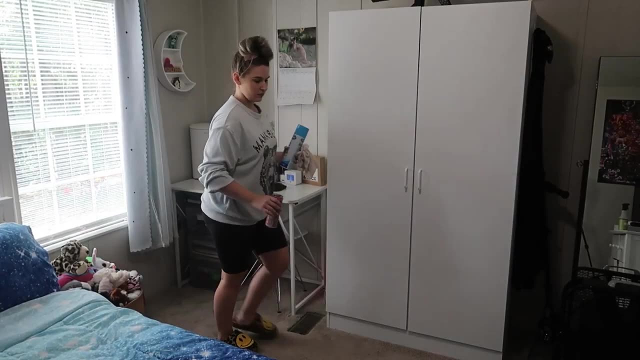 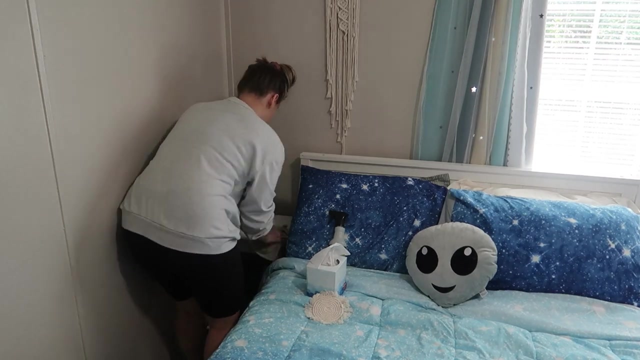 I spent a few hours deep cleaning- speed cleaning this room, and I was exhausted by the end of the day, but it was so worth it to finally get it done, So I'm going to vacuum one last time, and then I'm going to share a room tour. 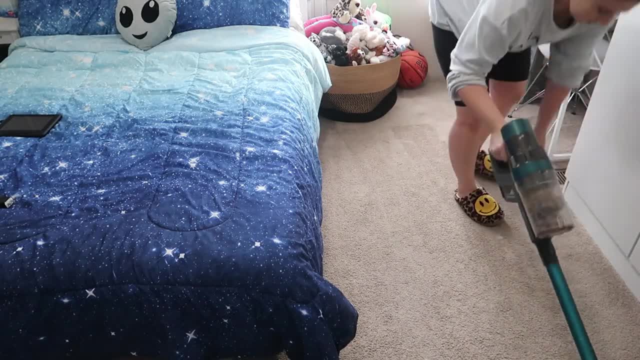 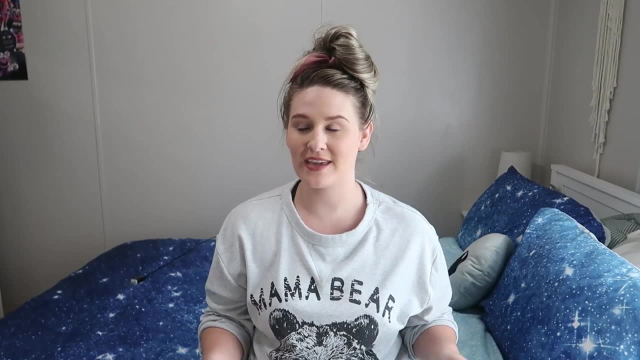 And I'm done. I had to stop 50, 11 times for my kids. The bus came, had to go get Bella off the bus. Jackson's awake, He's in his pack and play in the living room. Her room looks amazing It. 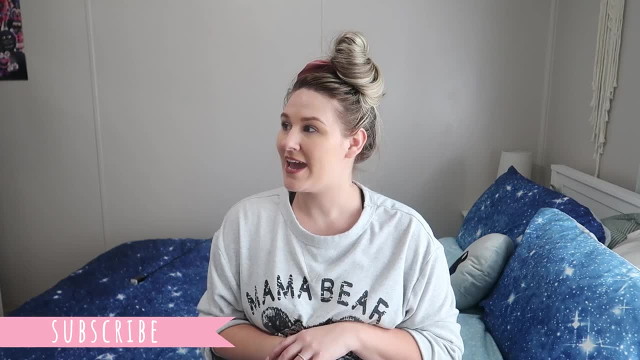 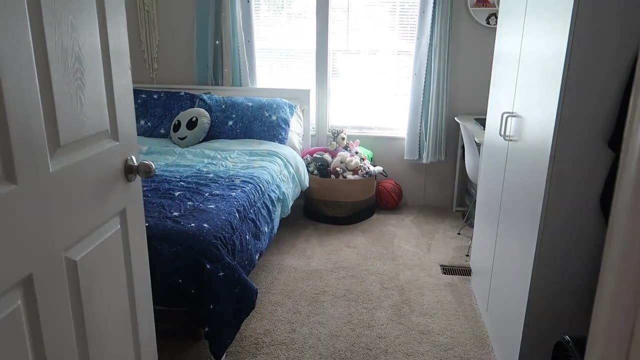 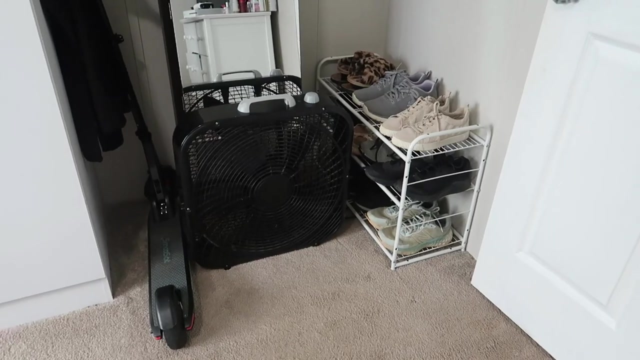 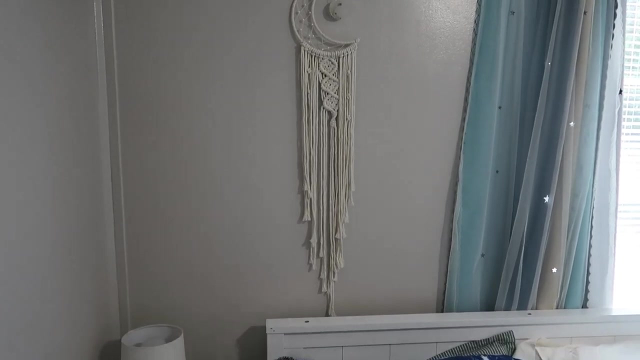 smells good, It's clean in here. It's dust free, So I'm going to go ahead and tour you guys around and show y'all the afters. So whenever she gets home from school today, I'm sure she's going to be so excited for her room to. 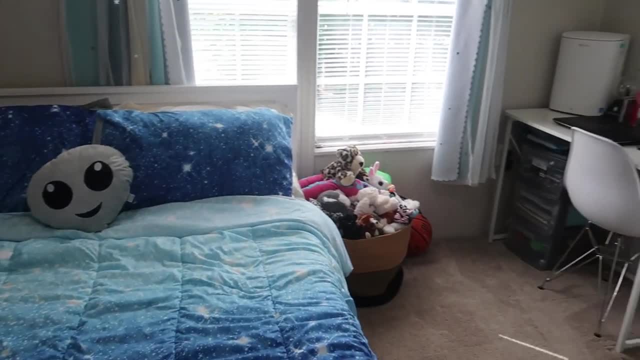 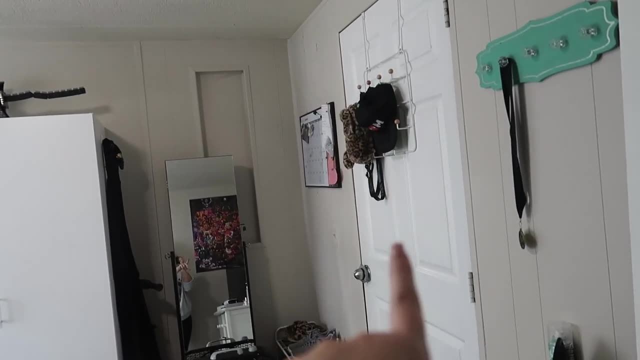 be back in order, And this is going to ease her anxiety. whenever she's sitting down at her desk and she's doing her homework and studying, She won't have clutter and mess all around her. So, to start over here, whenever you first walk in on the back of her door, that's just where she hangs. 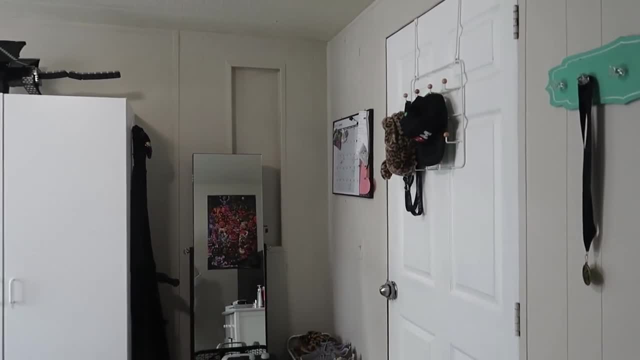 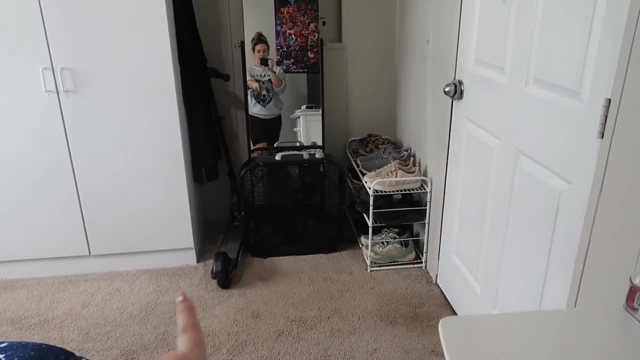 up her book bag and her purses. And then I have a drawer that she can put her stuff in. So I'm calendar here for her to write down all of her things, all of her activities and stuff. And then this is where I keep all of her shoes. She uses this fan at night, So she kind of turns it towards. 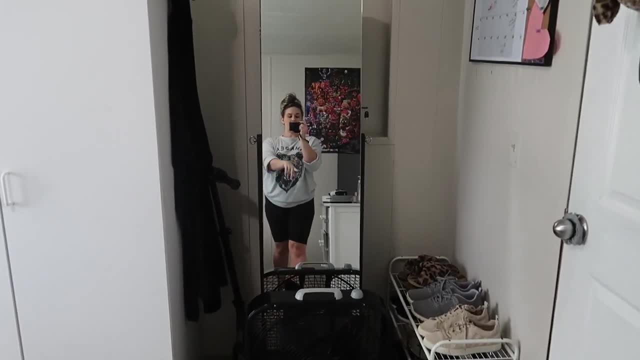 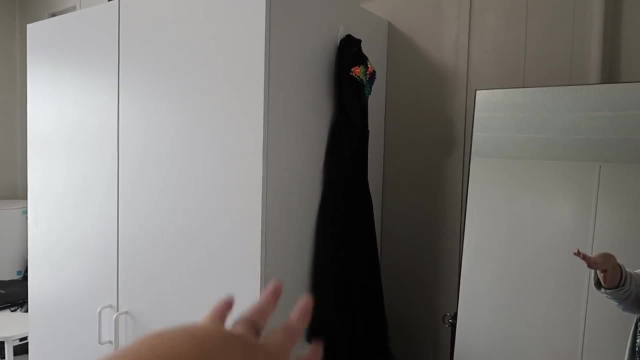 the bed, And then I just keep her electric scooter here Inside her mirror is where she keeps all of her jewelry and her scrunchies, And then I have a command hook on this. This is what I call her closet. That's just like her house robe. It's black with kitty cat ears And then on the top, 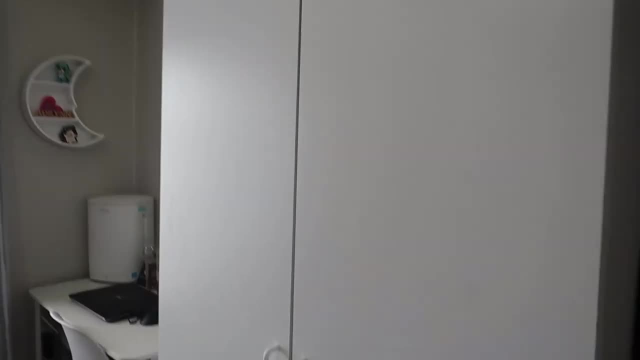 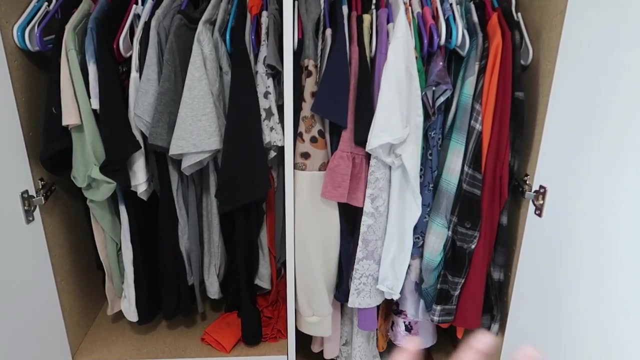 that is so much better. up there It's her favorite dragon And then I'll show you guys inside of her closet It looks so much better. She keeps her clothes on this pole here. This is mostly just like t-shirts and stuff, because we 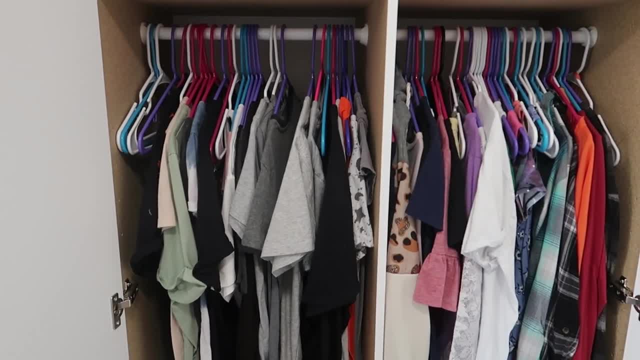 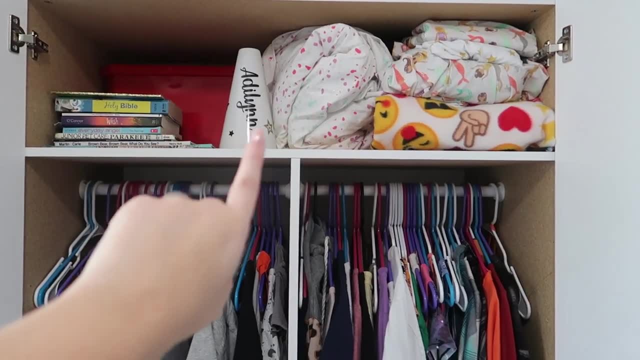 haven't had any cold weather yet, So whenever the cold weather comes, we will be getting out her winter jackets and her winter clothes On top. I have her Legos in the back. I stacked up her books here. That's her megaphone from the last time she did cheer. And then I just have like an extra. 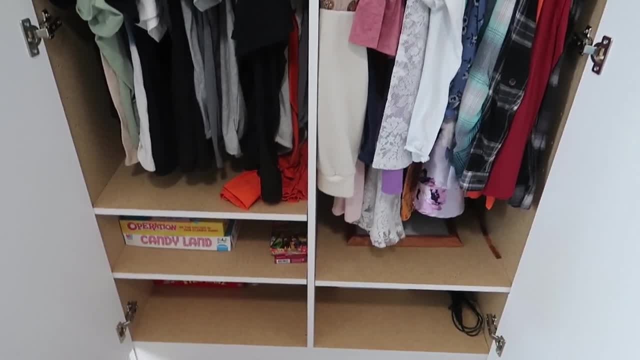 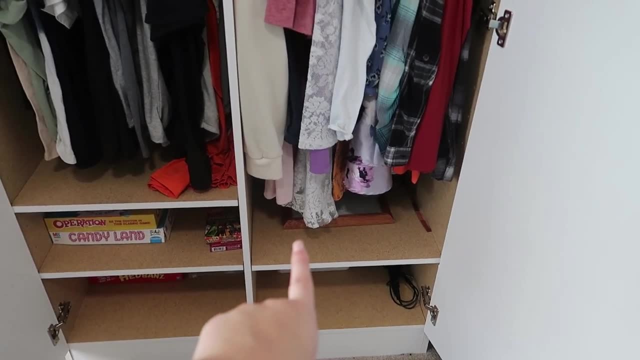 comforter and pillowcases and all of her sheets and stuff up there And then down here I just have board games and cards. She has like personal items down here And that's her microphone to her karaoke machine. This is so cute. This is something that she did with her pawpaw in 2013. And it's just. 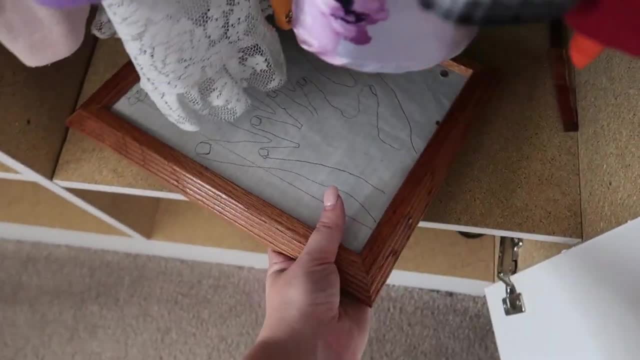 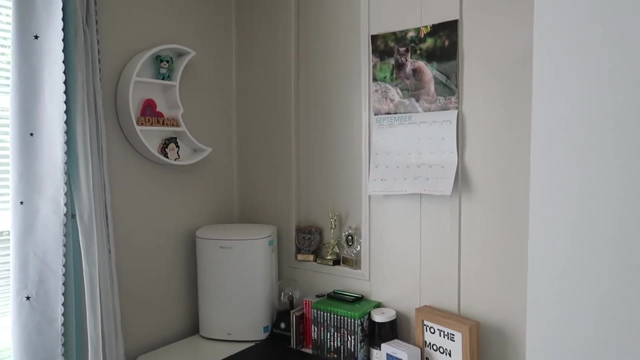 super special because her hand was so tiny and that's her pawpaw's hand. So that's just a little keepsake of hers. And we got this closet from Lowe's And then to the left of her closet is her desk. So she has a kitty cat calendar, her moon shelf and I'll just let her decorate her. 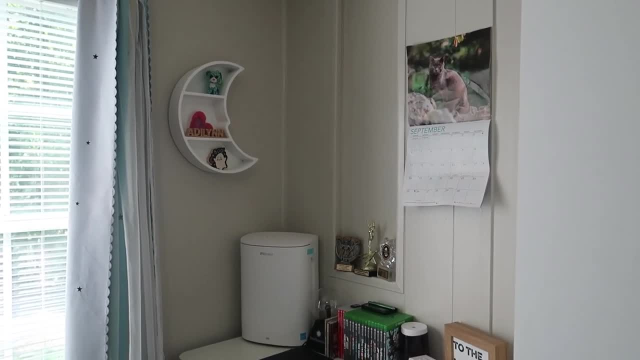 room any way she wants to. You guys, I don't come in here and make it look super aesthetic. This is the way she wants her room. So she just has a few little things up here. This is her air purifier. It just cleans the air. 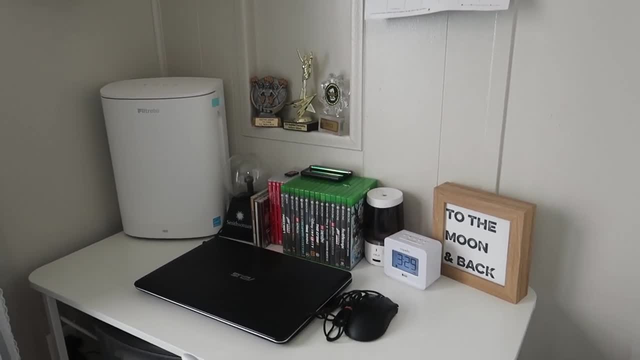 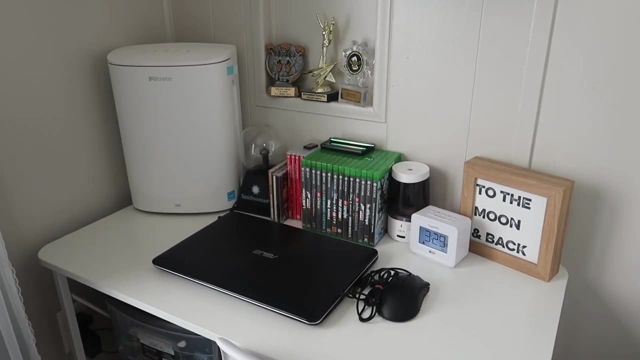 And then I just put like her games and CDs here. She usually just listens to music on her tablet or the computer, So she doesn't really have very many CDs. She had a ton of kids bop CDs that I just decluttered out of here. I'm going to be passing them down to Arabella, So she has some. 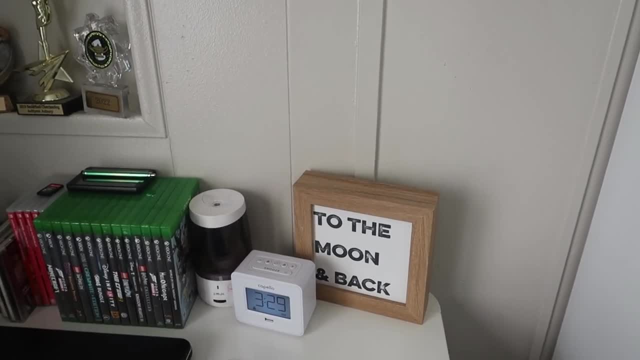 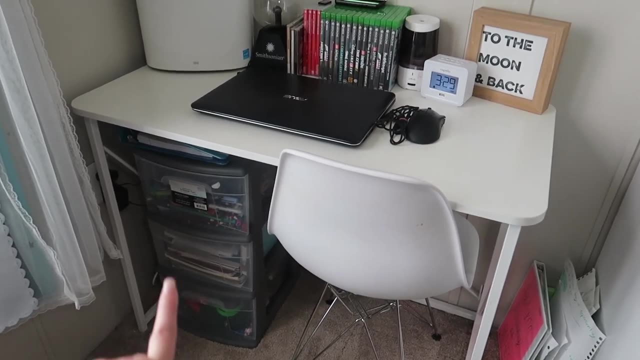 cheer trophies. Her room is galaxy themed, So we did a to the moon and back. This is actually my laptop. I gave it to Adeline because I don't really use it anymore ever since I got my new computer Over here. since this desk doesn't have any storage, I have this. I'll show you guys what's. 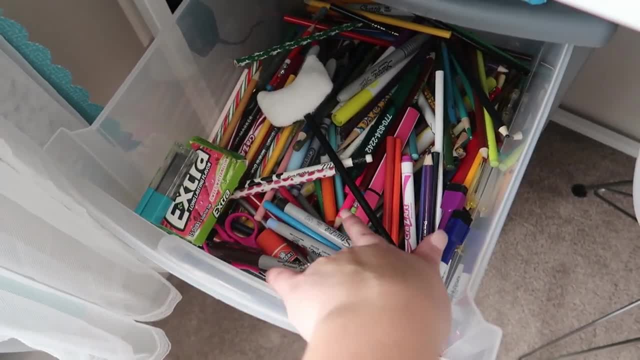 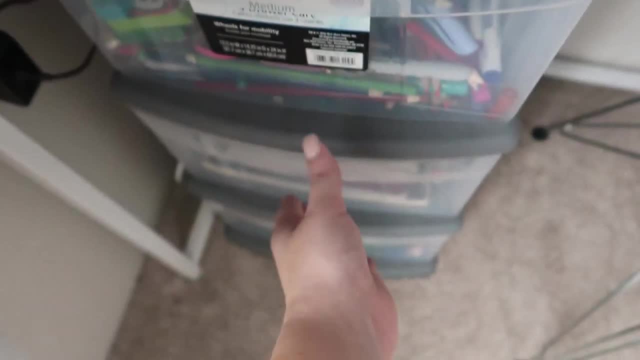 in here. So in this top one, this is where I keep all of her pencils And markers and scissors and glue. She has some gum and some extra lead for her lead pencils sitting right here. She's an artist so she's got lots of stuff like that, So I just dedicated a. 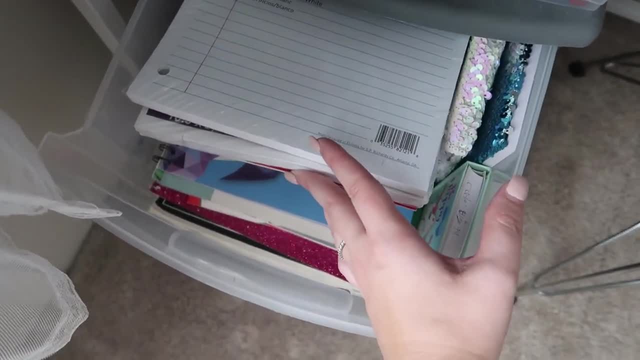 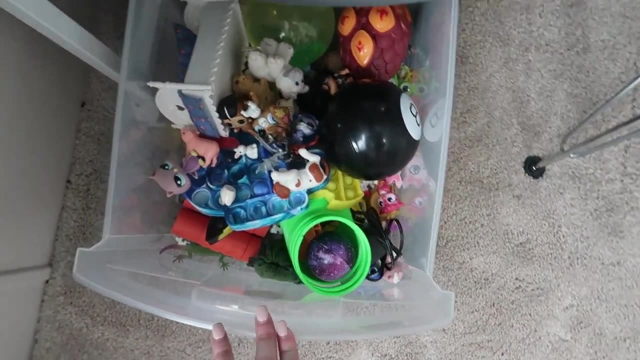 whole drawer to markers and colored pencils and stuff. This is coloring books and paper and her journals and diaries. Down here is what I call her toys. She doesn't play with toys very much. Also, I need to get my vacuum and kind of like go in the cracks of her carpet, So I need to do that. 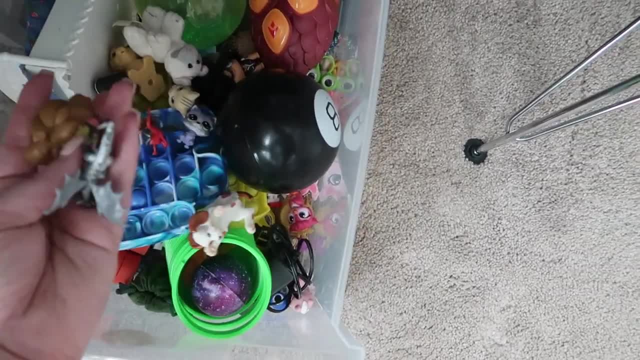 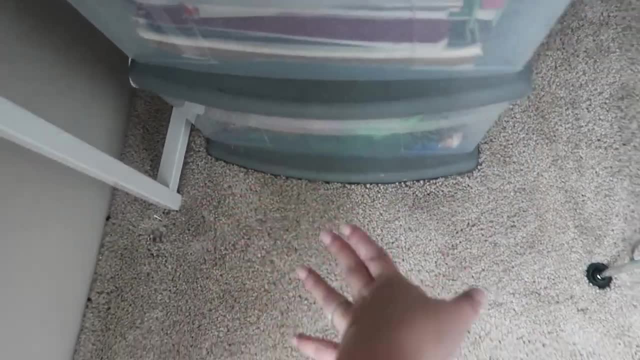 today too, still. But anyways, this is where I keep all of her like small little things like this. I don't know what it is about kids her age and the little tiny toys, but I just dedicated this whole bottom shelf to the little tiny stuff. I just have this tote full of her stuffed animals. 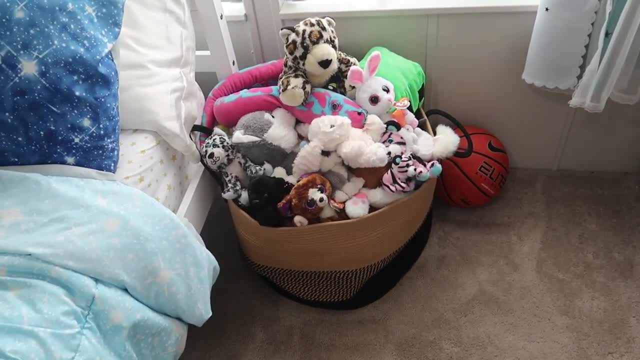 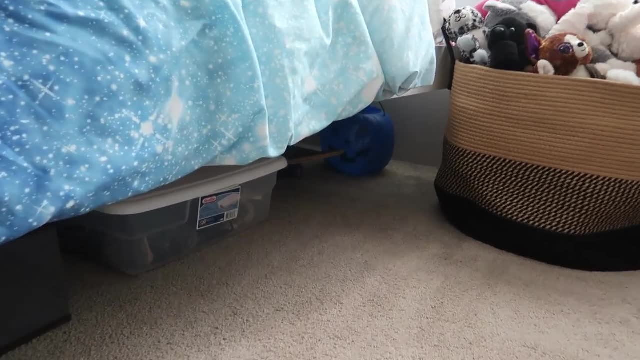 They were all up underneath the bed in a tote, but I feel like she can't really enjoy her stuffed animals when they're stored away, So I wanted to put them all in this basket, and then I have her basketball beside it. I'll show y'all- underneath her bed too, y'all I put in the 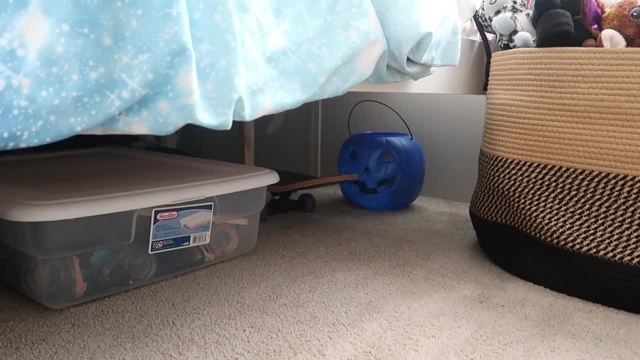 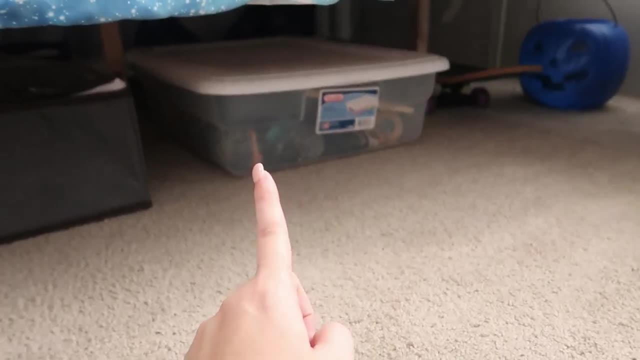 work today, So that's her Halloween bucket. It is September, so Halloween is coming up, So I don't really want to put that up, but usually it gets stored away in storage. We have a storage box building outside. She has her skateboard. This is a tote that just has like pieces to like her. 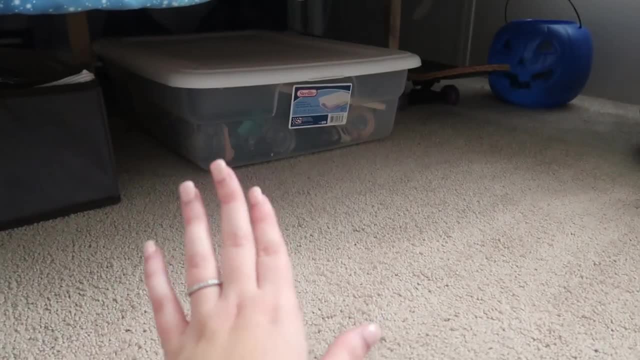 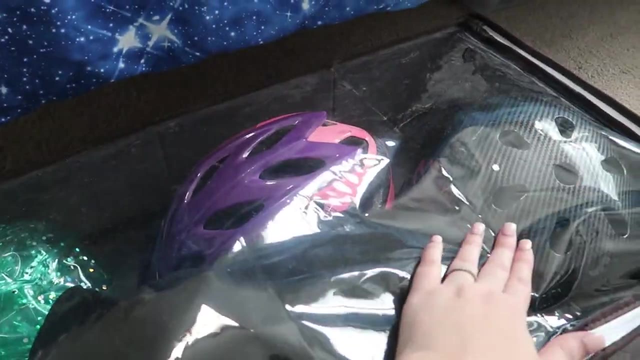 video games, like infinity stuff- I think it's called, but just like stuff like that is in there. Just her things, okay. And then in this one here, this is like a summer float Summer's over Her bike helmet, skateboard helmet and her skateboard gear And I need to wipe this down. 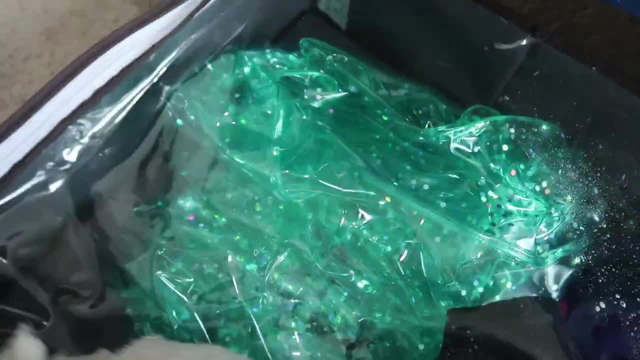 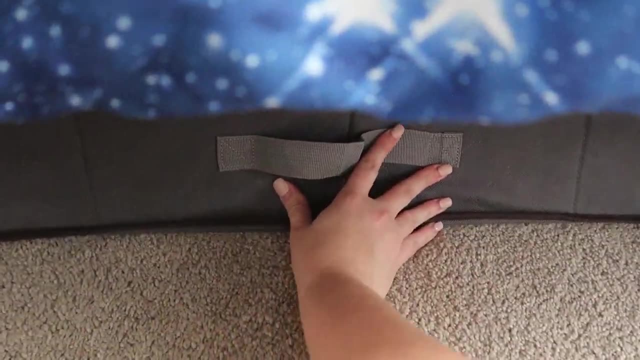 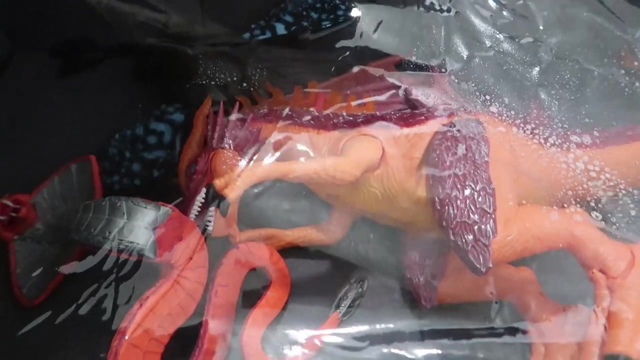 actually. so I'm about to do that. This is where I stored all of her like larger things that don't fit over there in the small toys. This is where I keep all of her dragons. So she has quite the collection here going on of like dragons and stuff like that. So just any like larger toys. I'm just 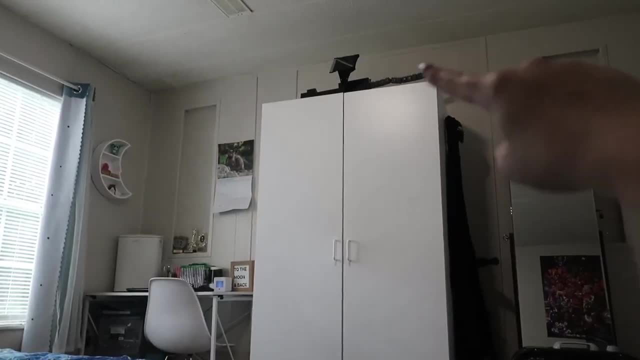 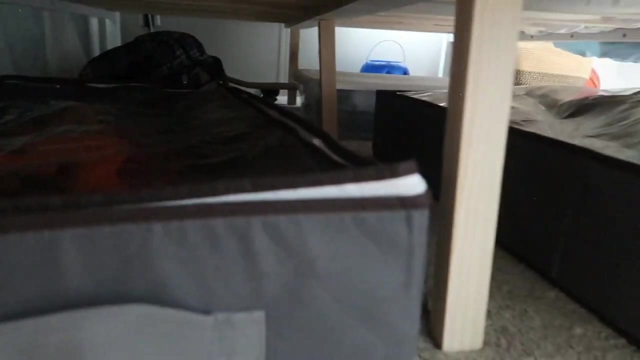 going to store it in this tote under the bed, And of course we have her large dragon, her ender dragon, up there, And then way back there in the back behind this tote, is just her overnight bag. So that's really all that's up underneath the bed, And then over here on this side of the room is 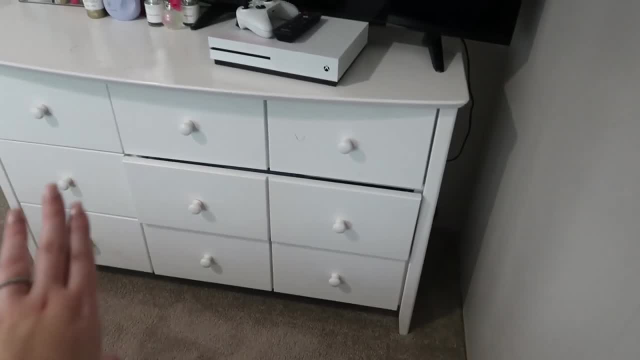 her dresser. So I cleaned out underneath her dresser and I'm going to have her go through all of her clothes when she gets home from school today And pull out anything that's too small or she doesn't want. She's going to do that in her. 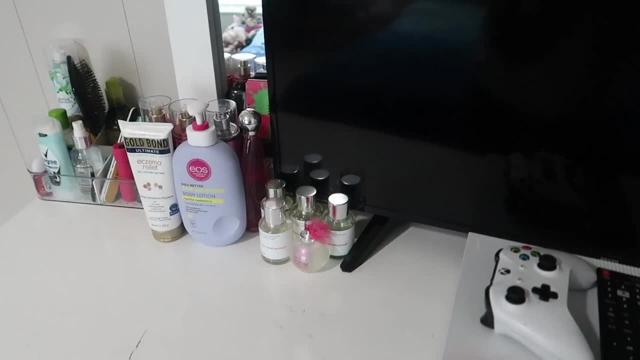 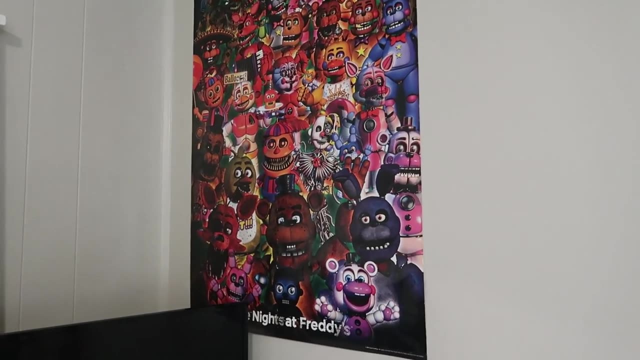 closet as well. I don't like to go through her clothes, because she's old enough to pick and choose what she wants to keep, So we have her Xbox and her TV. She has this poster that we recently got from Five Below. It's like Five Nights at Freddy's or something, So that's what. 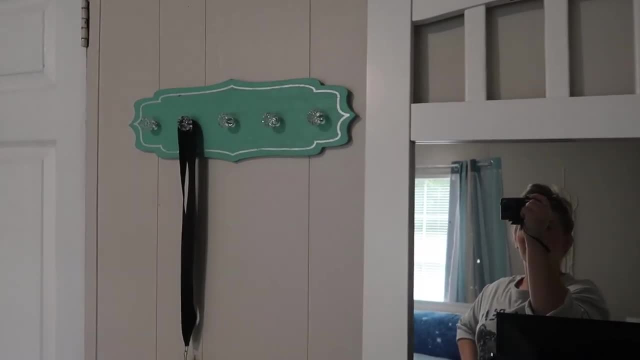 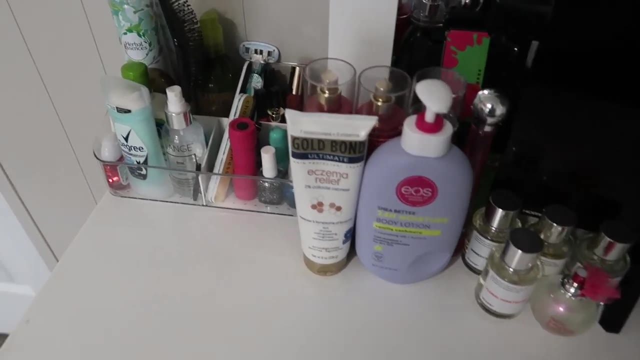 she likes. Over here I just have this turquoise. I don't really know what you would call that And, honestly, we could probably declutter that because it's not really serving a purpose other than being decorative right here And then right here on the top of her dresser. this came from Target. 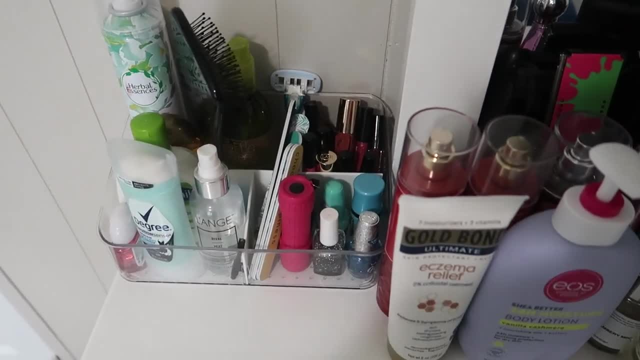 Dollar Spot for $5. And I just keep all of my clothes in there. So I'm going to have her go through all of her fingernail polishes, her nail polish, her hairbrush, her hair stuff, deodorants, things.